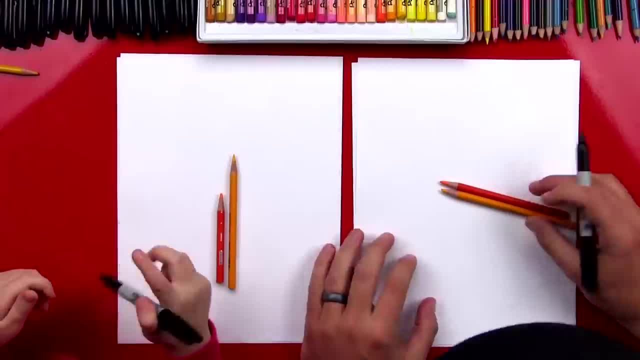 Yeah, It's going to be awesome. You ready to start? Yeah, We're going to use orange and yellow to color our candy corn at the end. Let's put that off to the side. We're going to use our markers first. 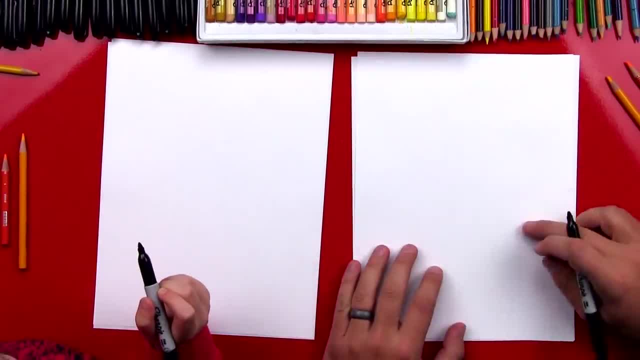 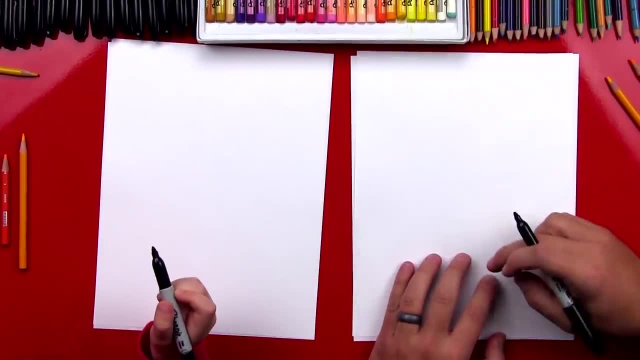 And the first step is we're going to draw an A with a round at the top, A rounded corner. So you don't want it to be a point, Okay. Okay, A candy corn is a triangle shape. Okay, Can you remember triangle? 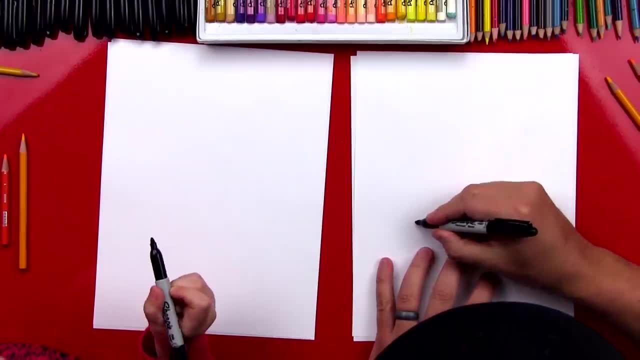 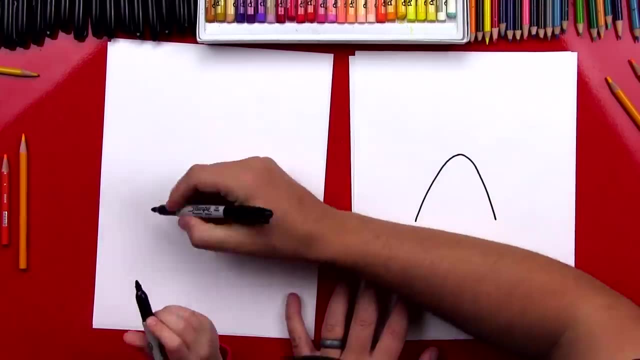 Yeah, Alright, so we're going to draw the A shape first. We're going to go up and then see how there's no point at the top, And then we'll come down like that: See it's round. So we'll start there, Go up and down Like an A shape. 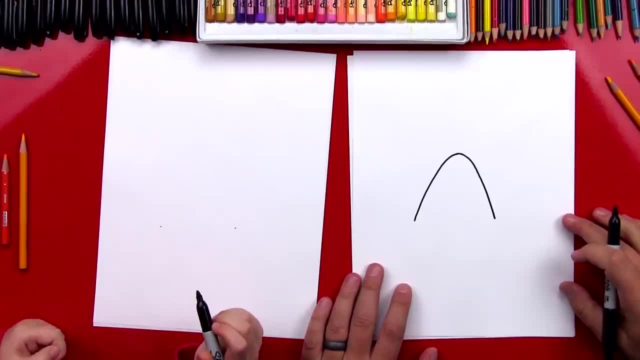 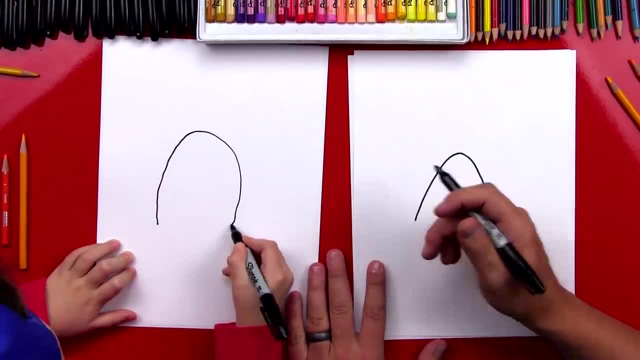 It's kind of like an upside down shape: An upside down U, An upside down U or an upside down V. Yeah, Good, And then. oh, that's a big one. I like it. Alright, are you ready to draw the bottom? 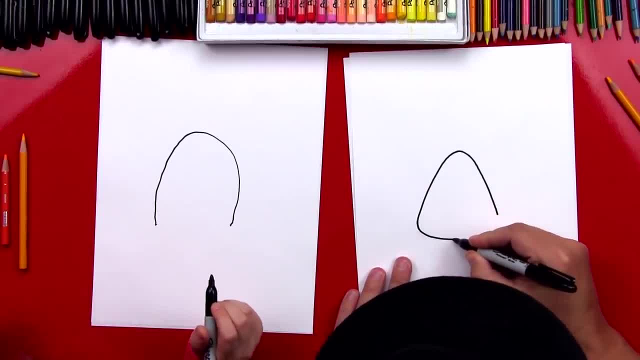 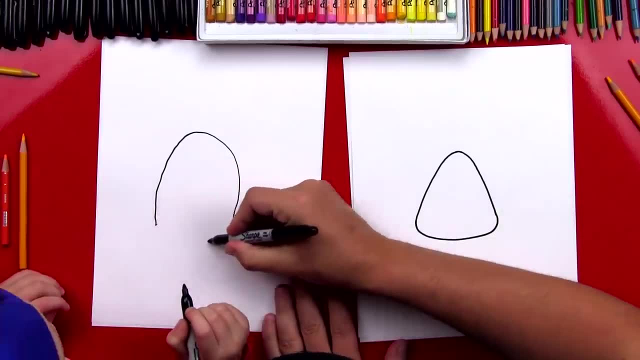 Yeah, We're going to connect the bottom with a round on this side and a round on this side. See how the corners are rounded. Yeah, Okay, let's connect and we'll leave the corners round. Yes, And then round in, Perfect. 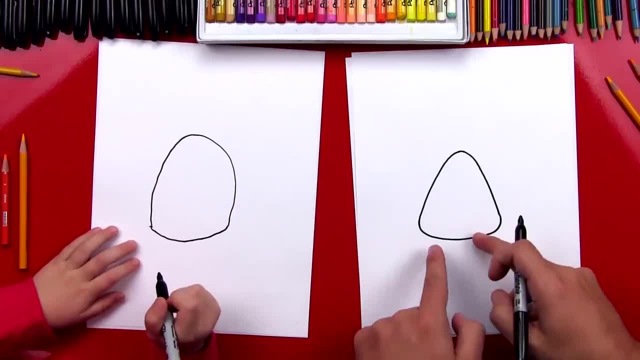 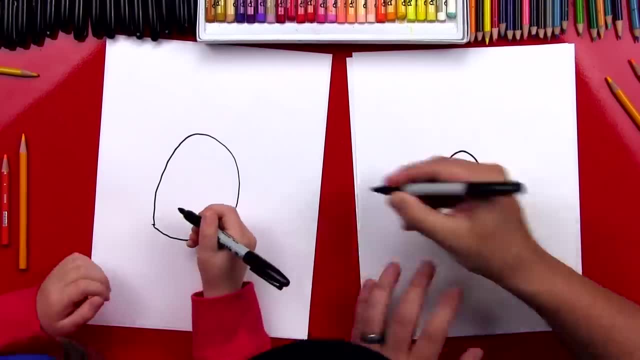 Alright, now that's the shape of our candy corn. What shape is it again? Triangle, A triangle. Let's draw the eyes next. Okay, We're going to draw a circle in this corner, So we'll draw a circle down here. 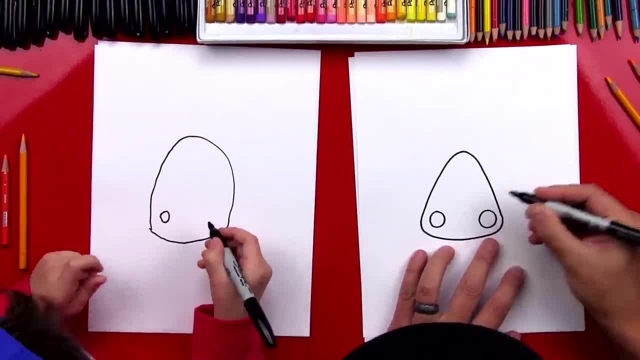 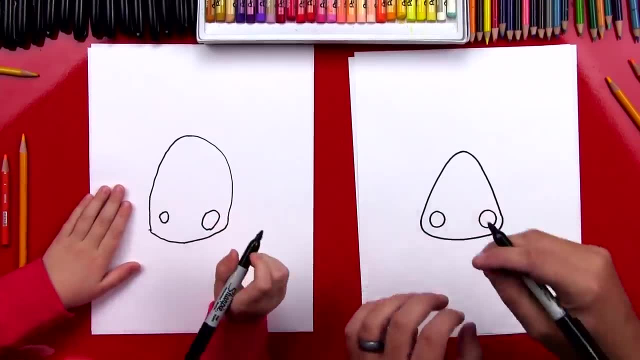 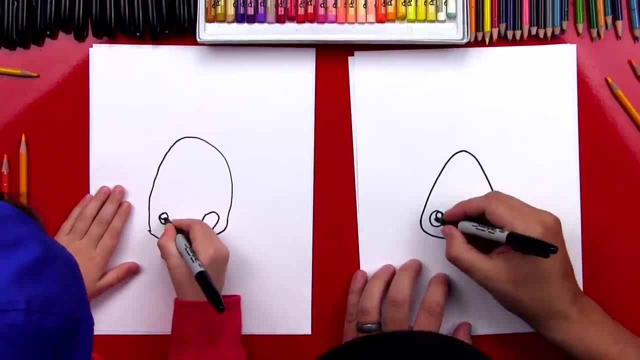 And then we'll draw a circle on this corner And we can make those the same size or different. And then we're going to draw little circles inside each eye. We're going to draw a circle in the top right And then we'll draw a smaller one in the bottom left. 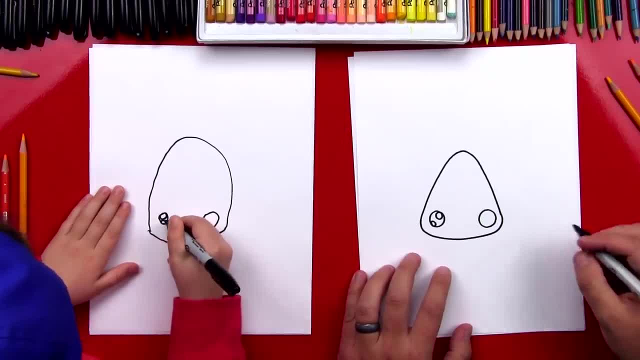 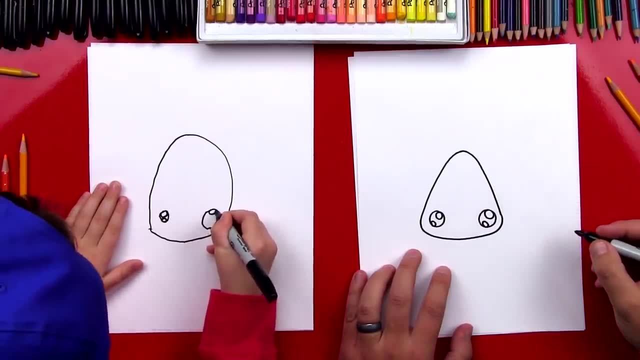 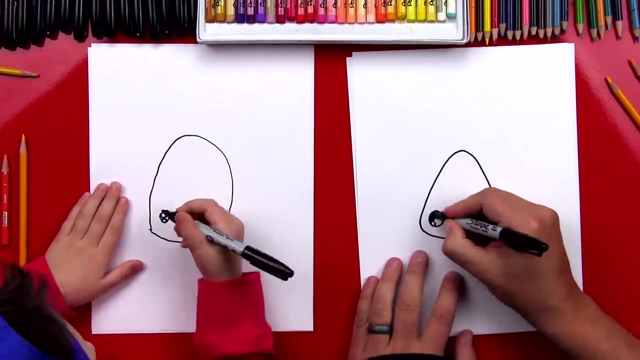 Do you have room? Oh, barely Good. And then let's do the same thing on this side: Circle on the top, Circle on the bottom, And then let's color in our eyes, But we're going to leave these little circles white. 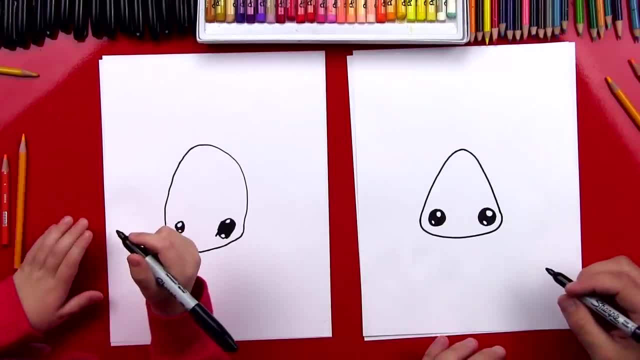 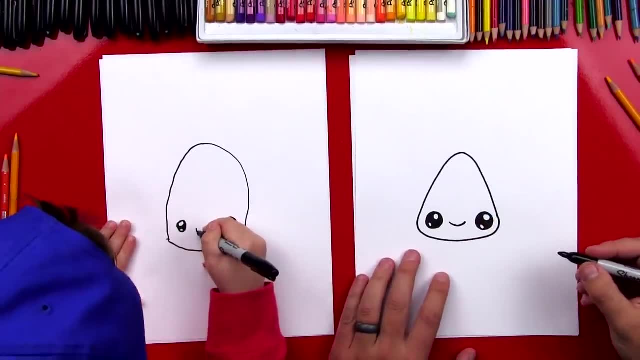 Good job, Austin. You colored your eyes. Now what should we draw? His smile, His smile, Yeah, Okay, we'll draw a little smile in between his eyes. Oh, I like it, It's a little one. Okay, now let's put our markers off to the side. 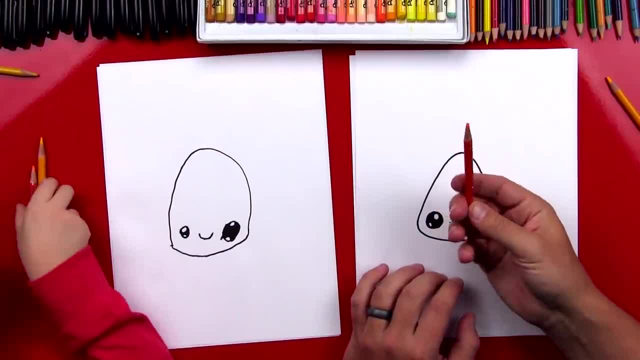 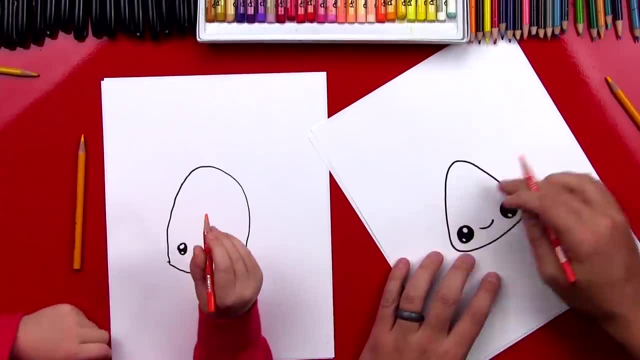 And we're going to use our orange colored pencil. Now, if you don't want to use colored pencils, you can use crayons or markers. Anything else, right? Yeah, Okay, let's draw the stripes on our candy corn. We're going to draw a line up here, up at the top. 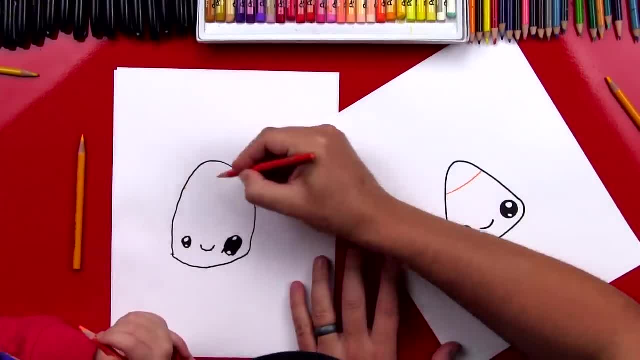 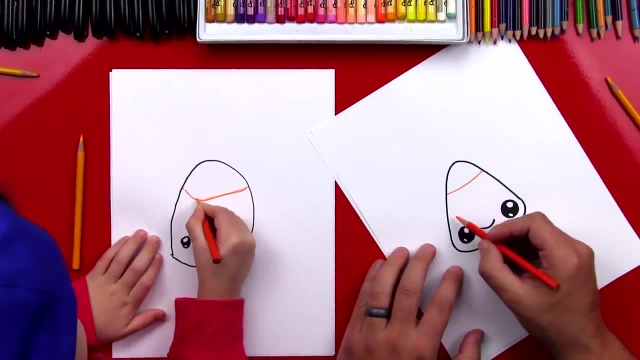 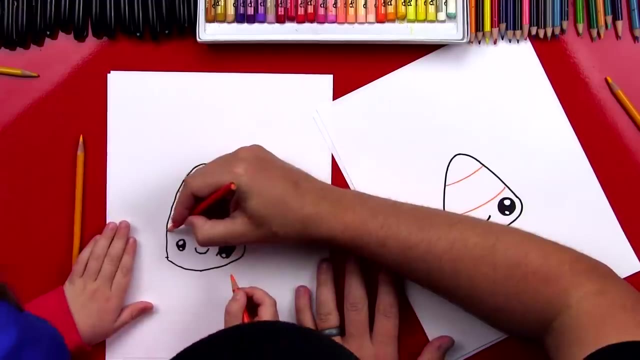 And I'm going to draw it curved, So we draw it right here all the way over to the other side. Good, And then let's draw one right above his eyes. We're going to draw another one right here, So we draw it down here to there. 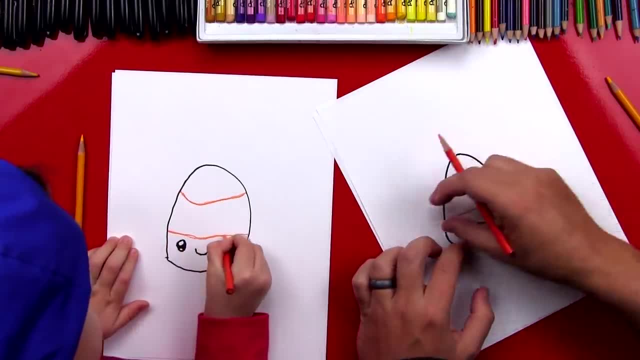 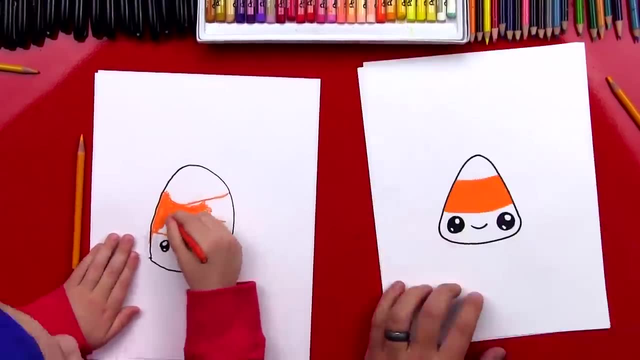 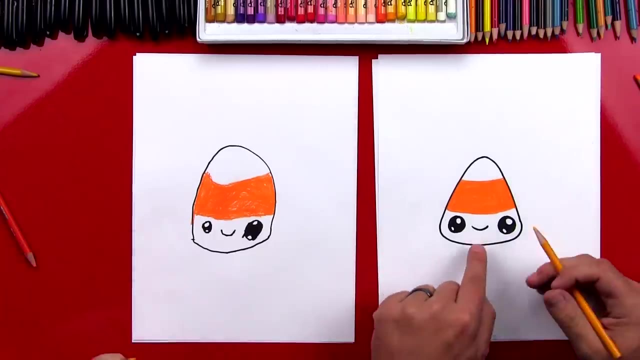 Yeah, Now we're going to color in his stripe right in the middle. Let's color orange and we'll fast forward. Nice, you did a great job coloring your orange stripe. Let's switch to our yellow And we're going to color the bottom stripe. 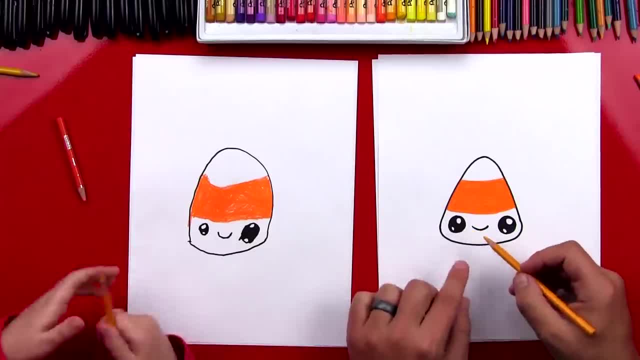 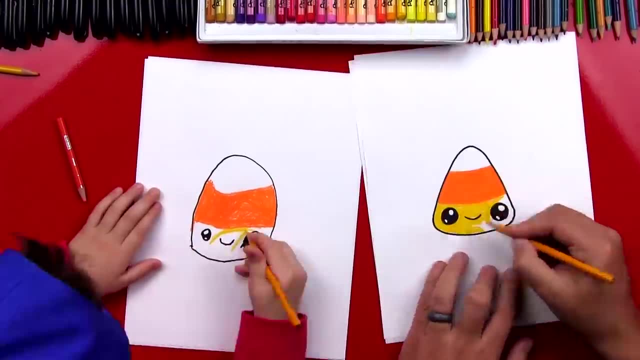 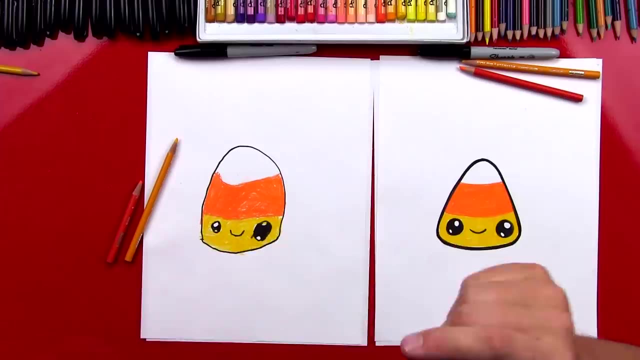 Oops, We're going to color the bottom stripe around his eyes. You ready to fast forward again? Yes, Let's do it right now, Austin. good job, man. You finished coloring your candy corn. Was that nice and fun? Yeah?